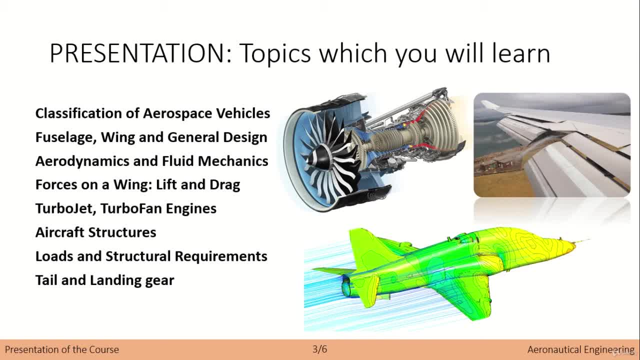 aerospace vehicles: fuselage design, wing and general design of an aircraft. aerodynamics and fluid mechanics. forces on a wing which imply lift and drag, basically turbojet, turbofan engines. also some structural conditions of aircraft, loads and structural requirements We will also study. 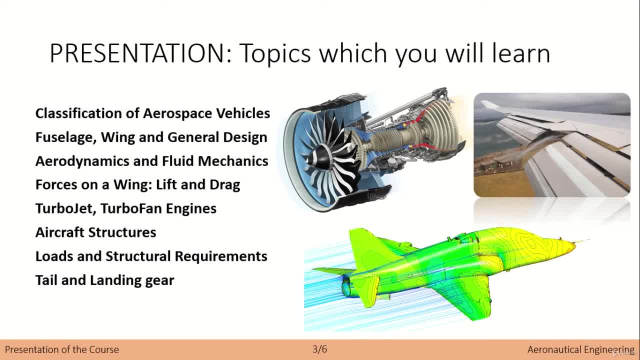 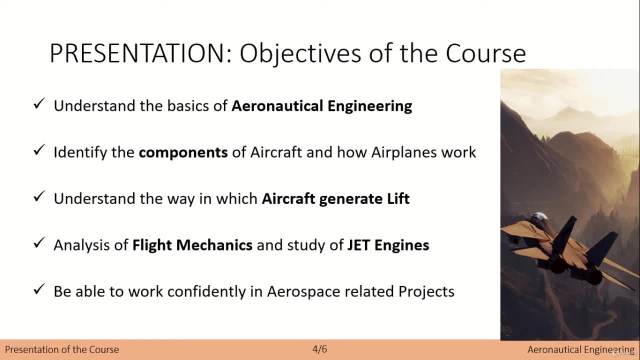 a tail and landing gear, and we will also cover some topics like performance and operational performance. So let's get started. The objectives of this course are actually to understand the basics of aeronautical engineering as a topic, identify the different components of aircraft and you will also actually learn how. 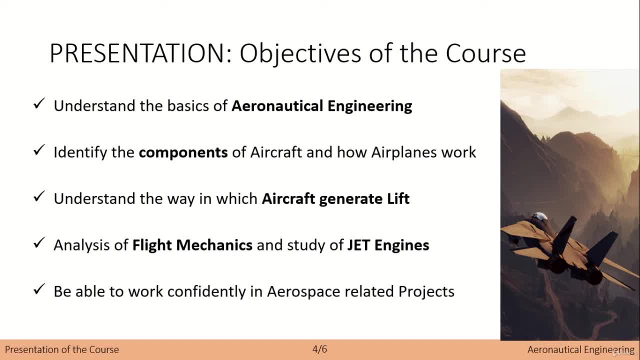 airplanes work and perform. You will also understand the way in which aircraft are able to generate lift, which is one of the key topics in aircraft engineering: analysis of flight mechanics and study of engines and specific aircraft. So let's get started And specifically jet engines and from this as an objective, my idea is that you will be able to work. 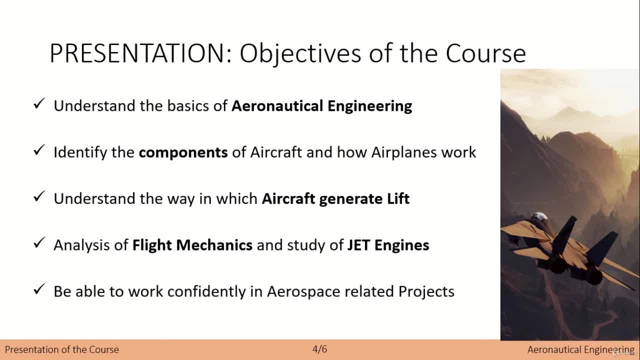 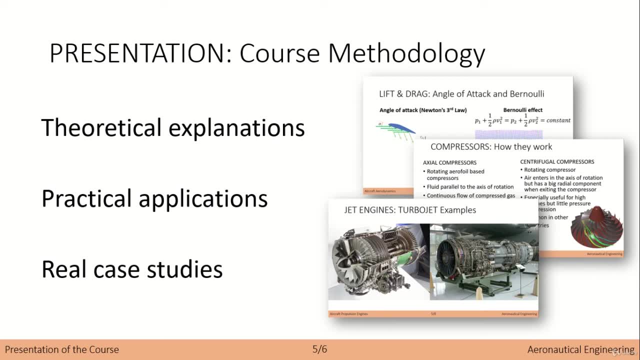 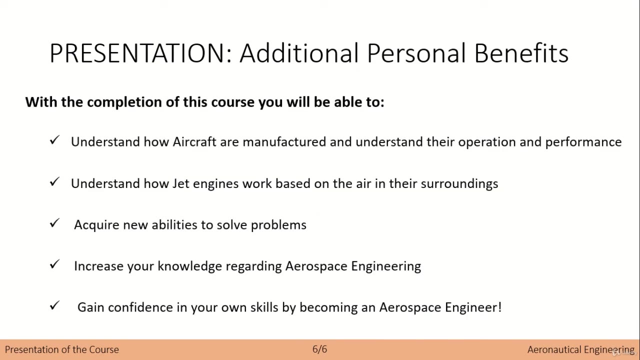 confidently in any project related to aerospace engineering. Now the course methodology is based on, first, theoretical explanations of physical phenomena, practical applications related to aerospace engineering and, finally, real case studies of different components, different elements that compose aerospace engineering today. Now you will also gain some additional personal benefits with the completion of this course. 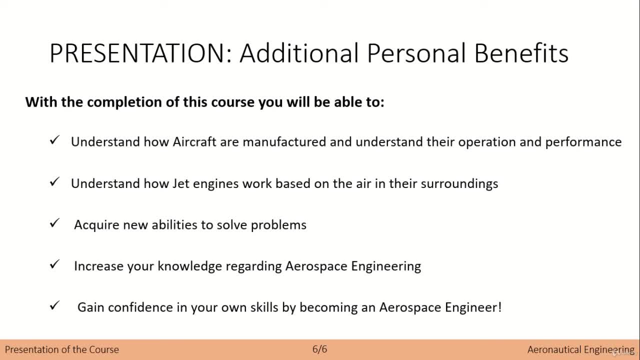 Okay, so you will be able, for instance, to understand how aircraft are manufactured and understand the operation and performance, for instance, limitations on the manufacturing regarding the design, etc. Understand how jet engines work, based on the air in the surroundings, and how they transform this air into thrust. Acquire a new ability to control the air flow. 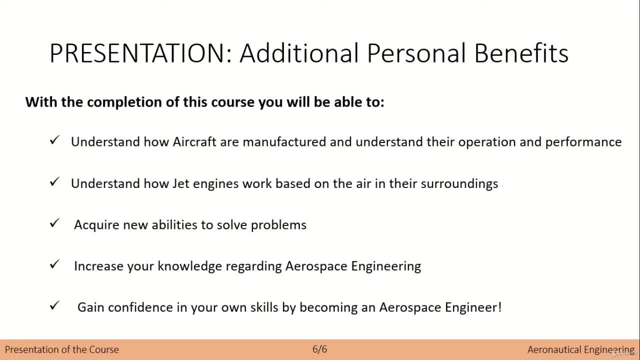 acquire new abilities to solve problems as a generic topic, also increase your knowledge regarding aerospace engineering and finally gain confidence in your own skills by becoming an aerospace engineer. To be honest, I am pretty sure that this course will cover most of the topics that you are. 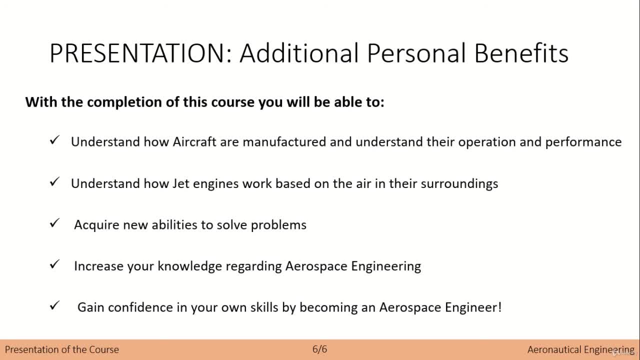 looking for in an aerospace engineering course. So, as always, if you have any doubts, if you want to make some comments or add some sections, then I'm completely open to do so and will listen to any questions. So welcome to this course.